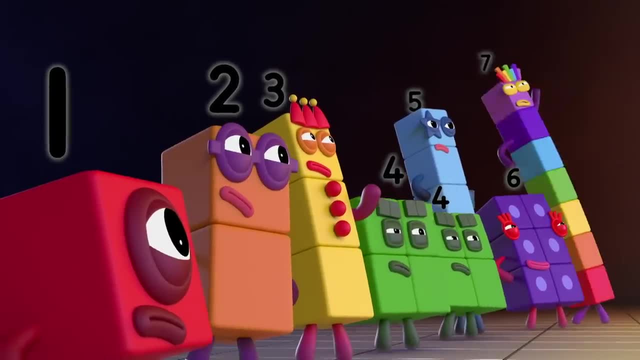 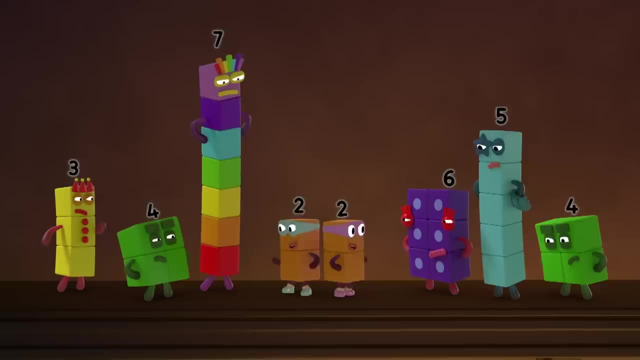 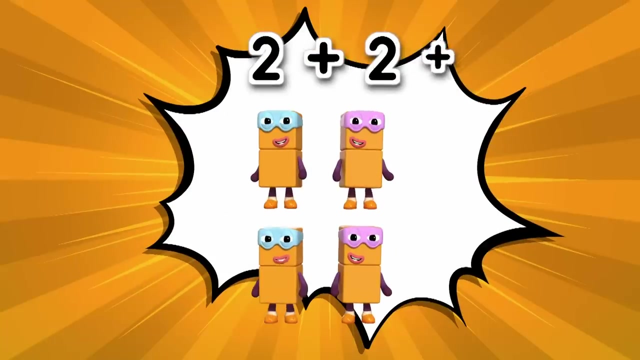 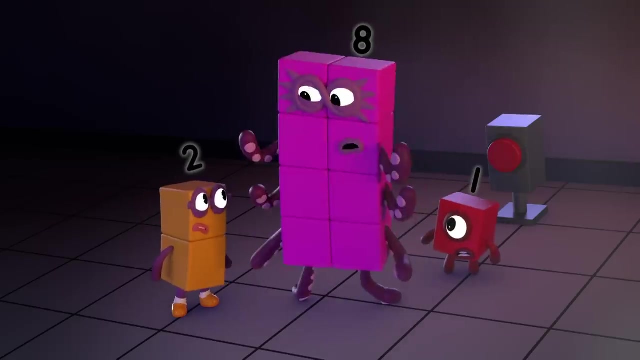 Stop right there. We have you outnumbered? Oh, Maybe so, But we've still got a trick or two up our sleeves. Two plus two plus two plus two equals Eight. Four terrible twos make one octonauty. You've met your match, Octoblock. 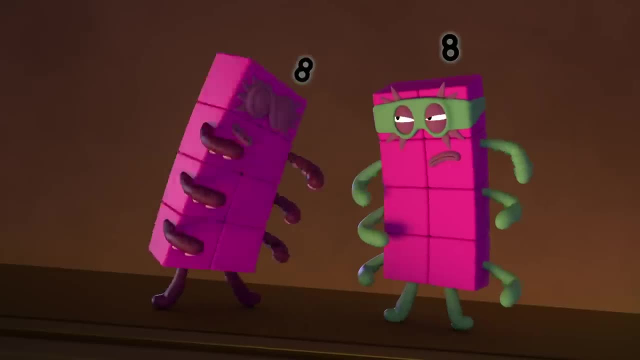 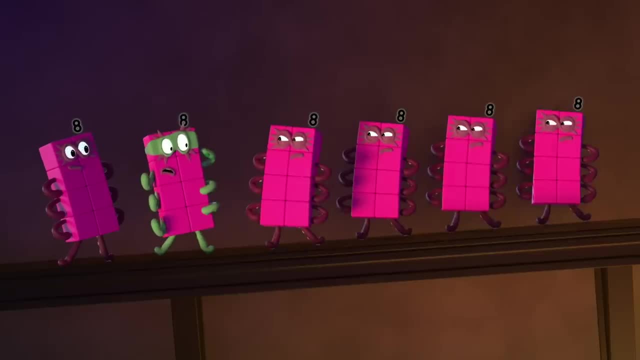 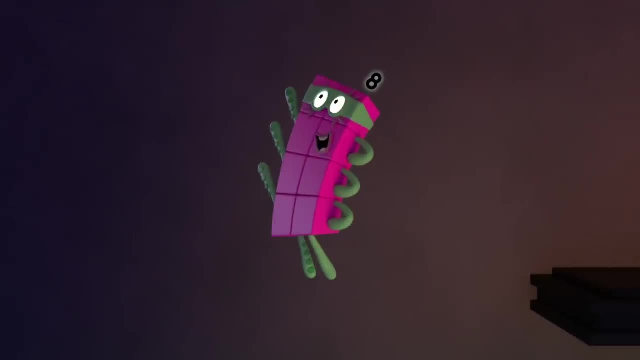 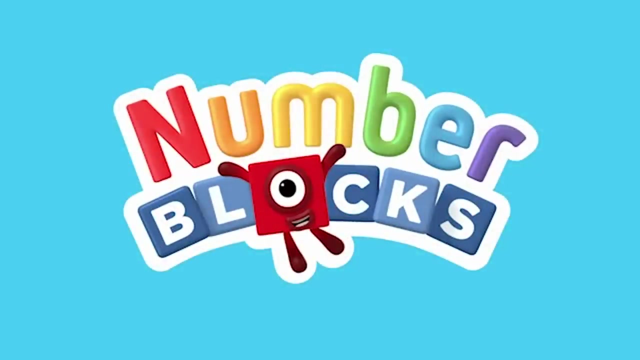 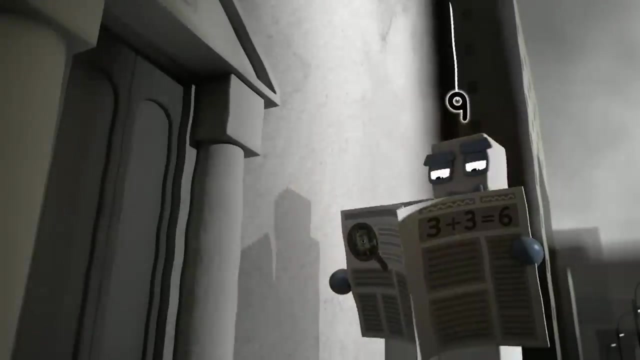 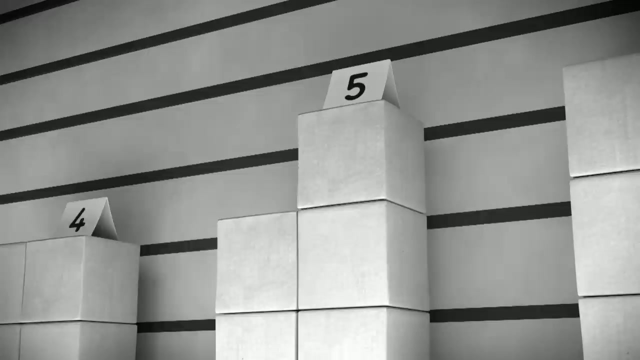 Eight, seven, six, five-four, three, two, one escape. Uh oh, Let's look at what we know. Clue one: The suspect had a flat head when standing two blocks wide, So it can't have been 3,, 5,, 7 or 9. 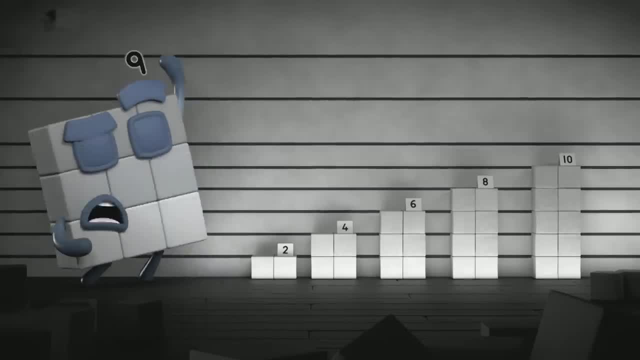 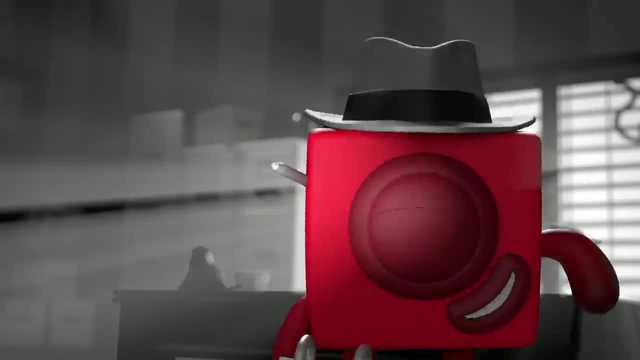 And it wasn't you, because you can't stand two blocks wide. 2,, 4,, 6,, 8,, 10. The suspect must be an even number. Bingo, And remember clue 2: The suspect was smaller than 9, So it can't have been 10. 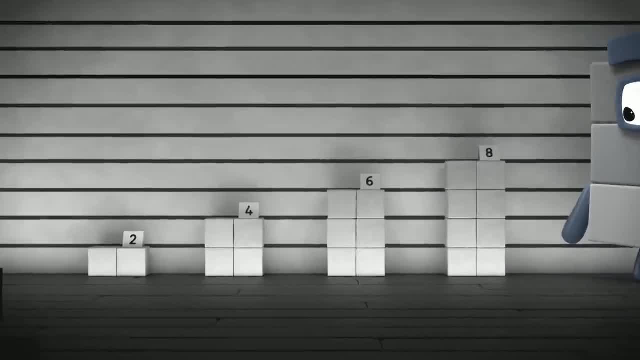 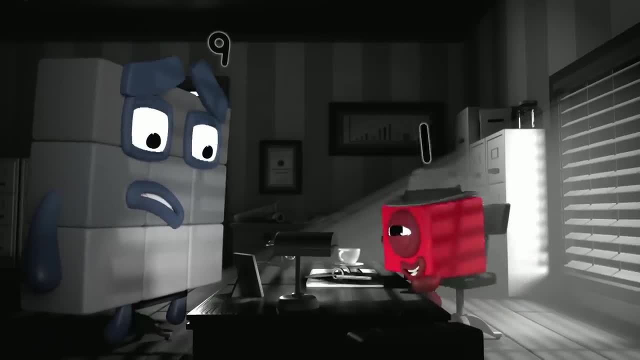 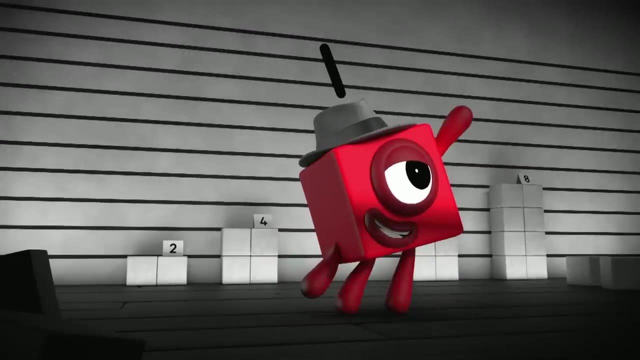 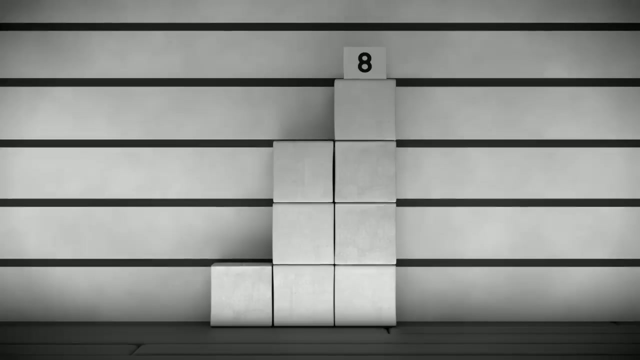 That still leaves 2, 4, 6 and 8. But which was it? Wait, There's one more clue. we nearly forgot. The suspect can make a step shape, Not 2 or 4 or 8, So it must have been 6. 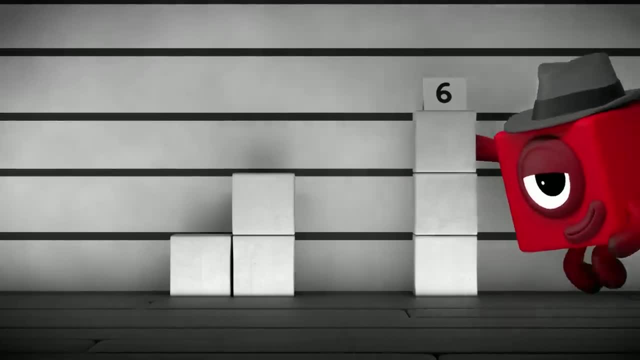 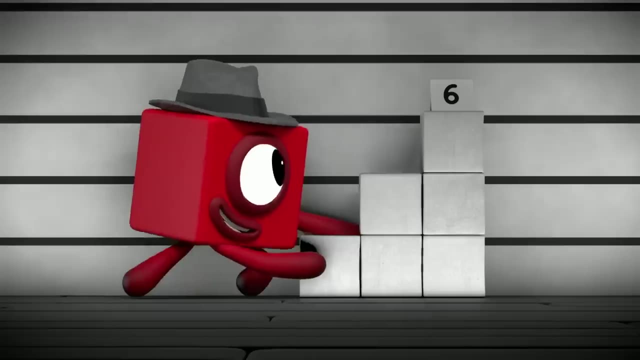 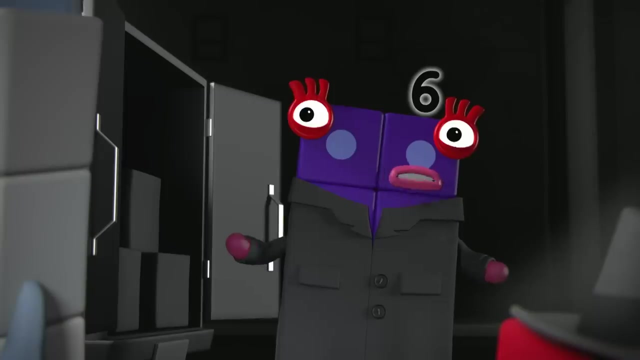 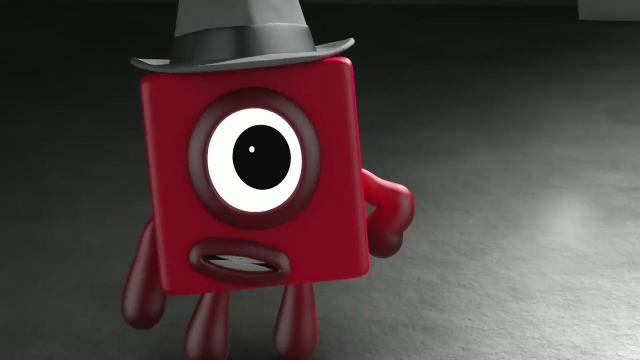 And who did we meet in the alley 3 and another 3 Equals 6. Stop Thief, You've got it all wrong. Oh, where to begin? I'm not taking these things, I'm moving them in, Moving in. Come up and I'll show you. 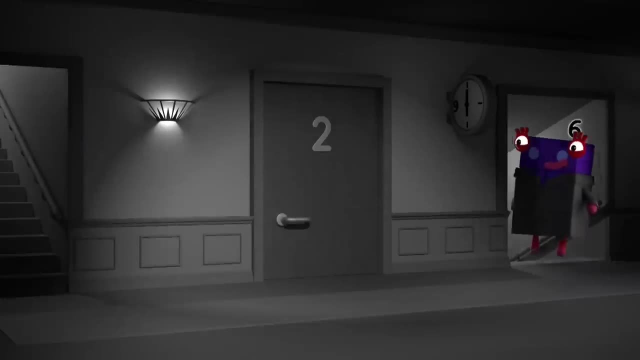 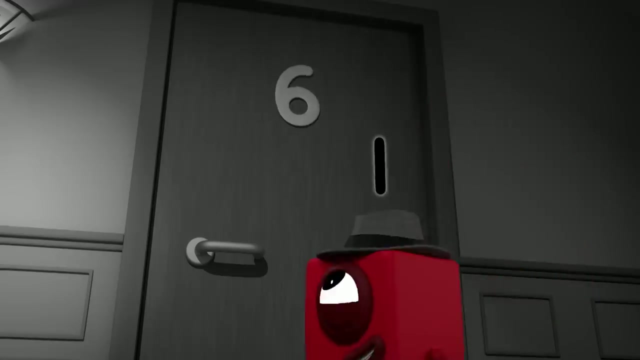 1,, 2,, 3,, 4,, 5, 9- Wait, 9 doesn't count. Come after 5?? This isn't apartment 9, It's apartment 6. Look, Number 6, turned upside down, looks like a number 9. 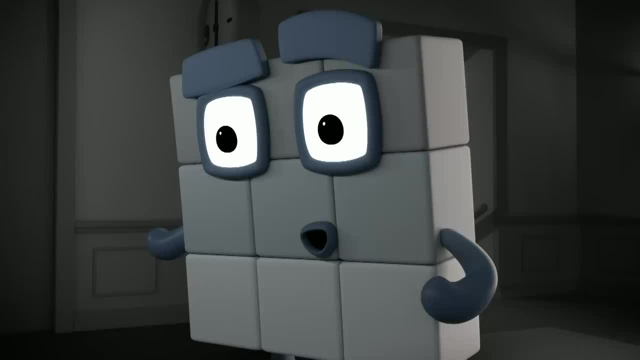 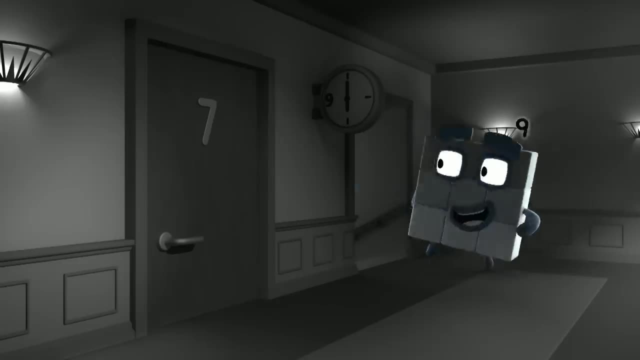 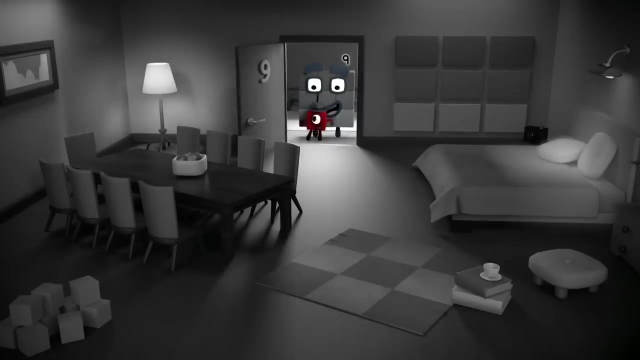 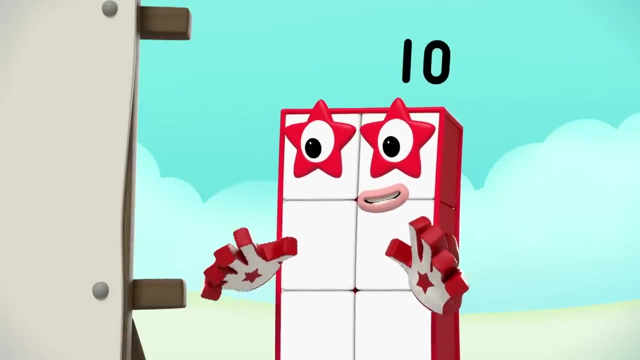 No one stole your things. 9- You went into 6's empty apartment, So my things must be Right where I left them. Case closed. 9- didn't count on us. we're the number blocks Six's house. Oh, I know how to cure hiccups. 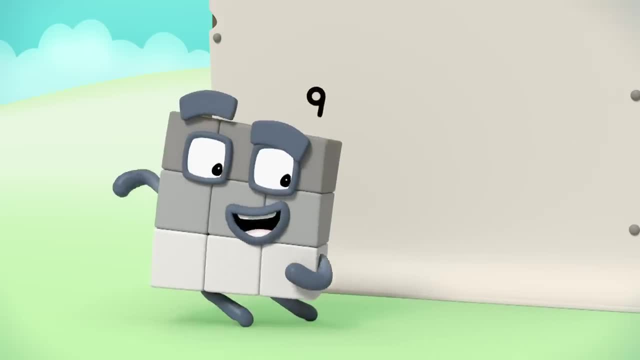 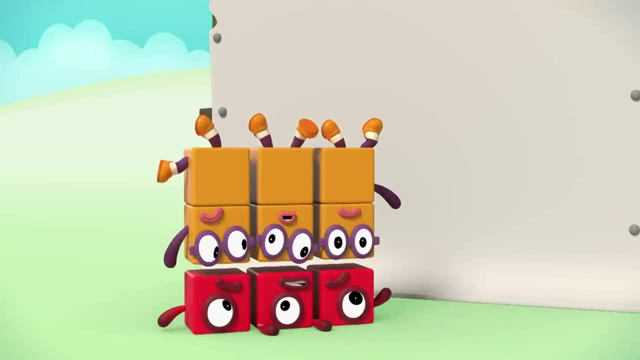 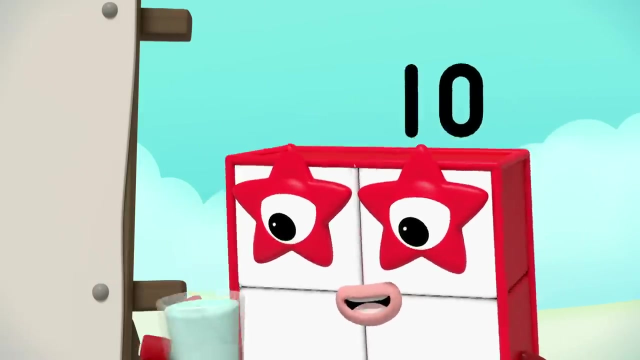 You stand on your head. Huh, Hick, Huh, Huh, Ha, ha. I think it's working, Ah, Hmmmmm, Hang on. I know another one. Drink a glass of water backwards. Drink Harder than it sounds. Harder than it sounds. 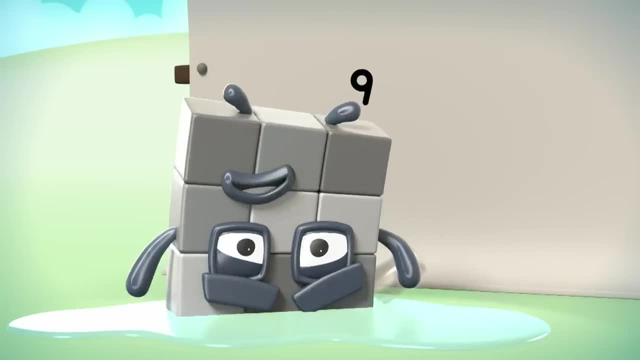 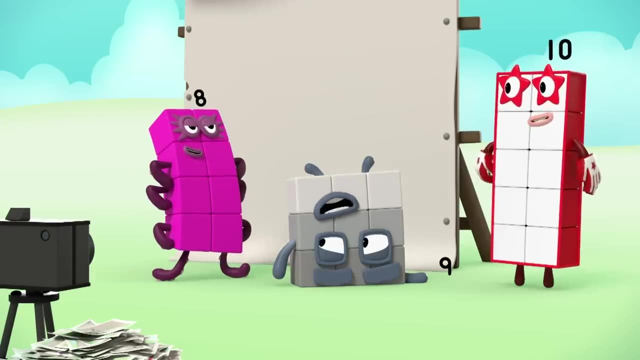 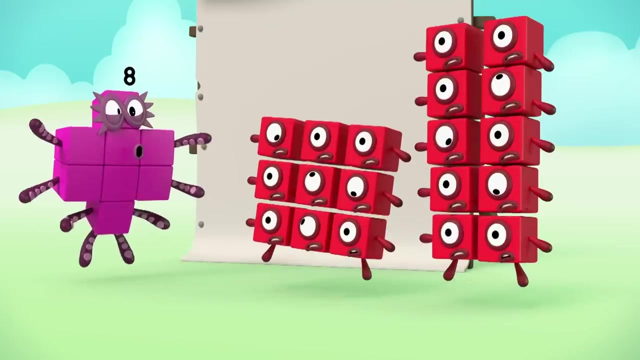 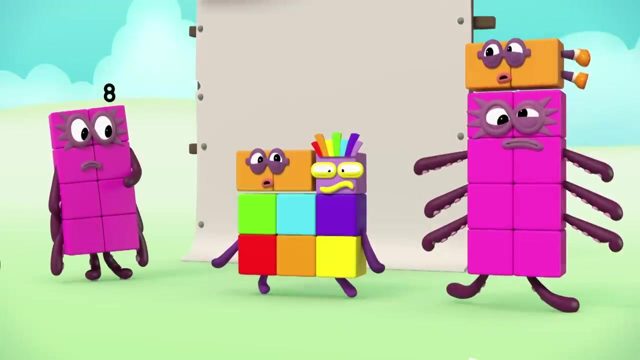 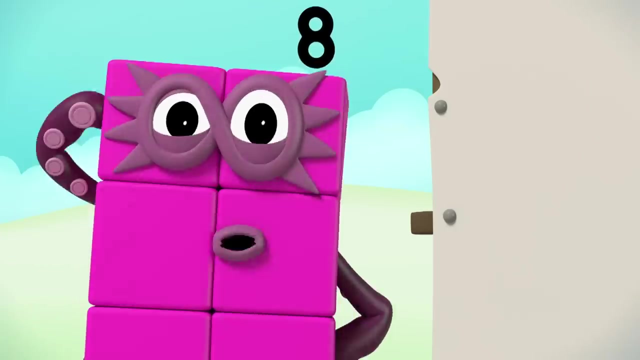 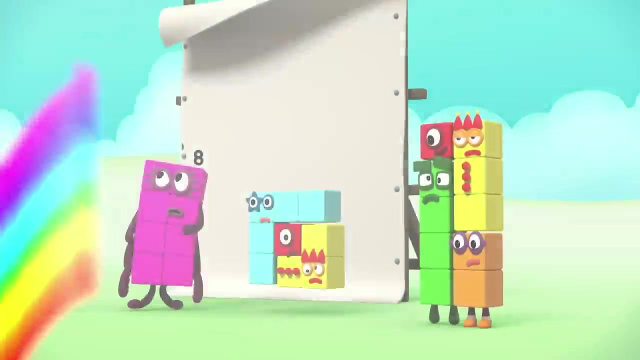 We need help. Have no fear, Octoblock is here. He's got hiccups. I know what to do, Octoblock- Sorry, That usually works Hiccups. Don't worry, I've got this. Lucky, lucky, lucky, lucky, lucky, lucky, lucky. 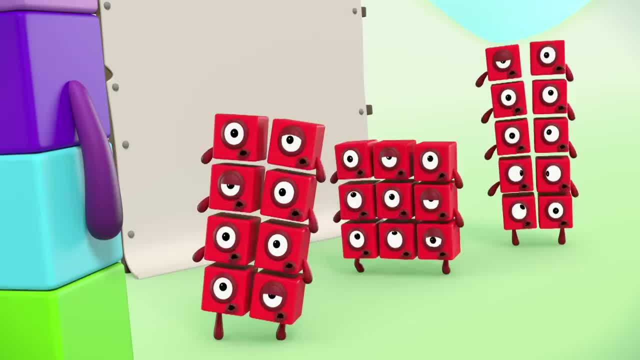 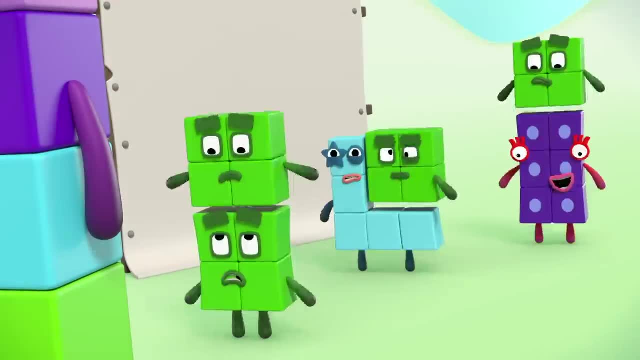 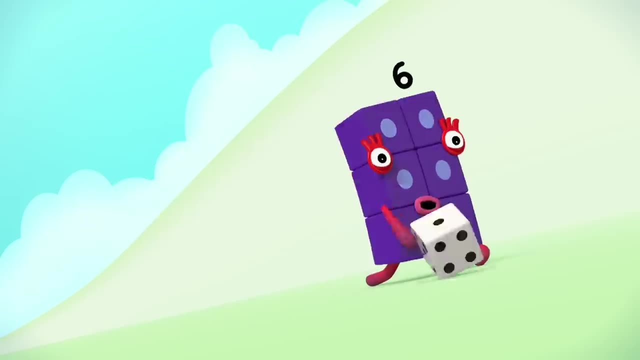 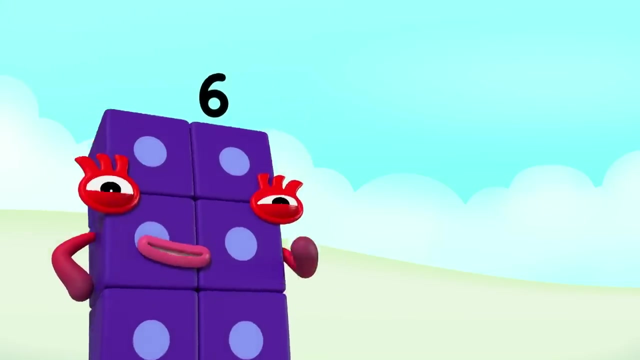 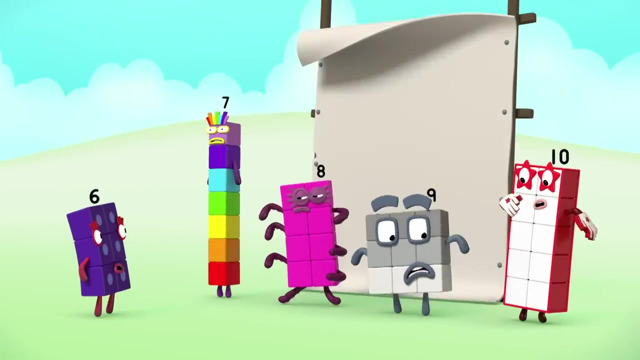 Help. Oh, I tried that Out of my way, Coming through, Got six hiccup cures for you. Let's roll Six. Cure number six: it is Boo, Boo, Boo, Oh, Oh, Oh Oh. 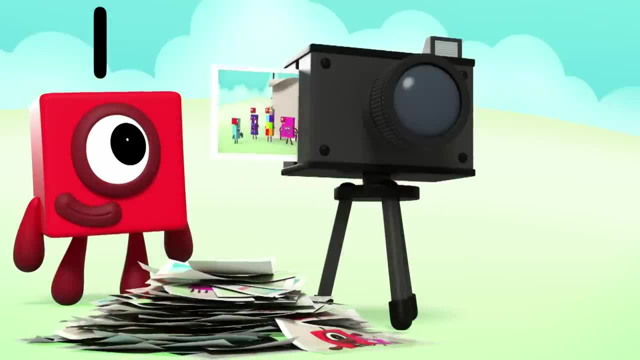 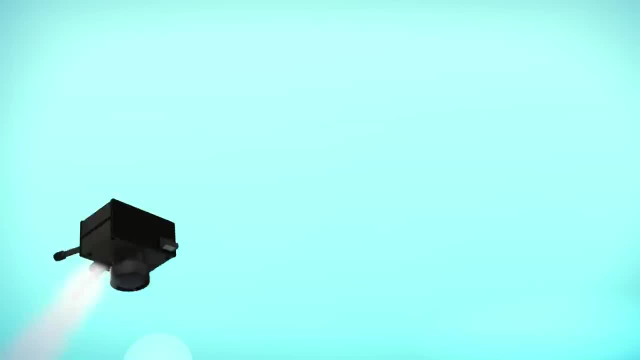 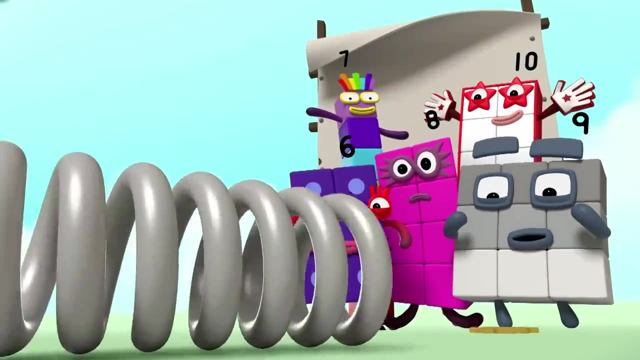 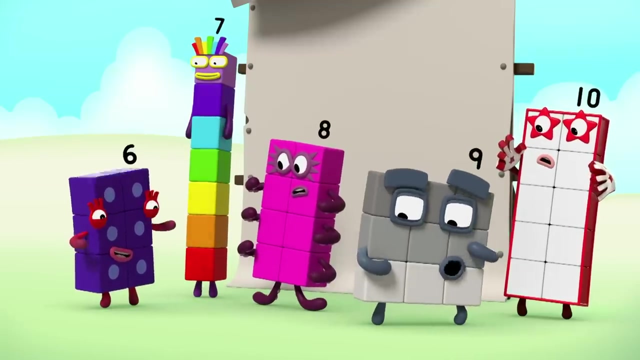 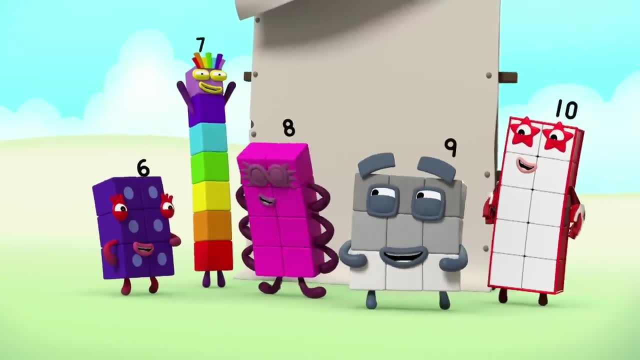 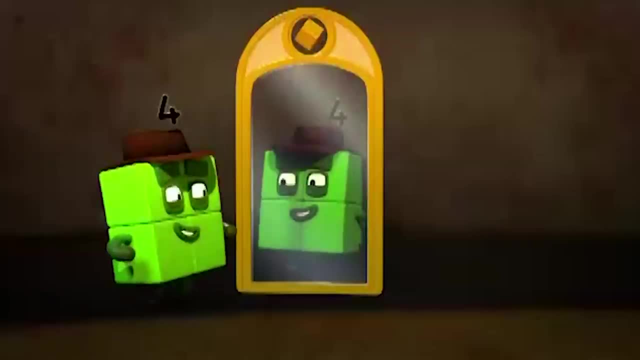 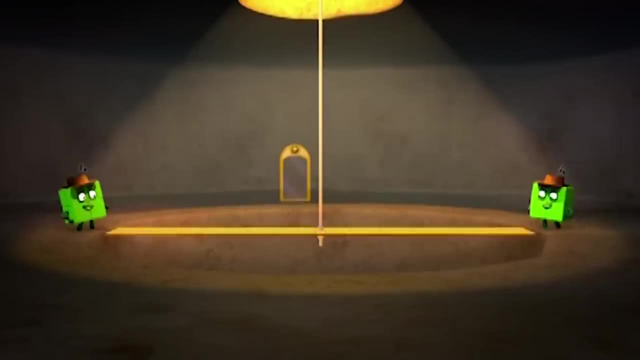 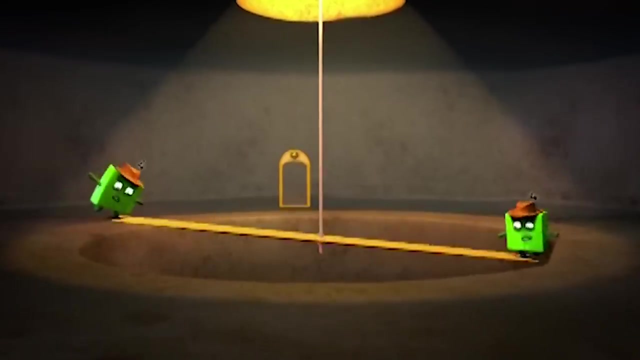 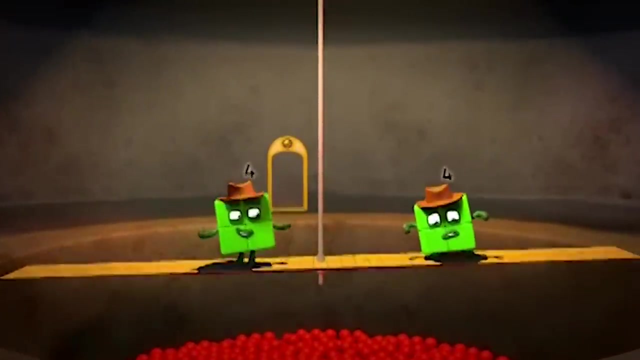 There's something there, Ah, something there. You can count on us with an OtterBox. Need some help. Four: You take that sign. One, two, three, four. now Keep going, Keep going And double up. 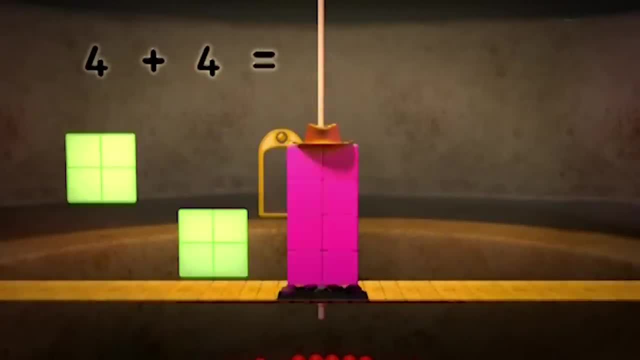 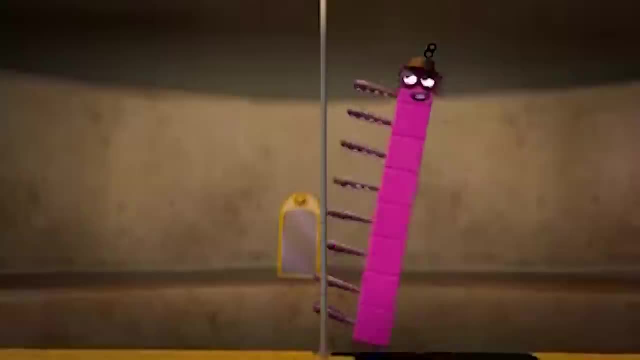 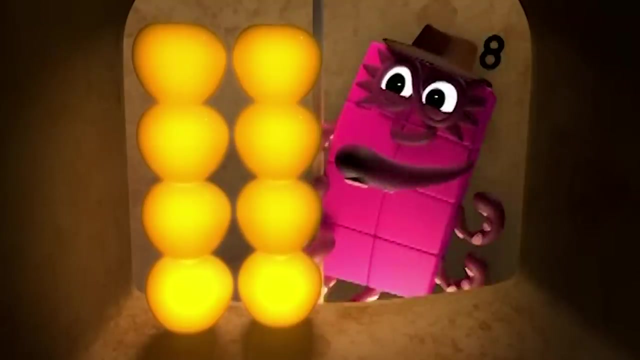 Four plus four equals eight Octoblock climb. One, two, three, four, five, six, seven, eight climb. The golden delicious One whoops: One, two, three, four, five, six, seven, eight climb. 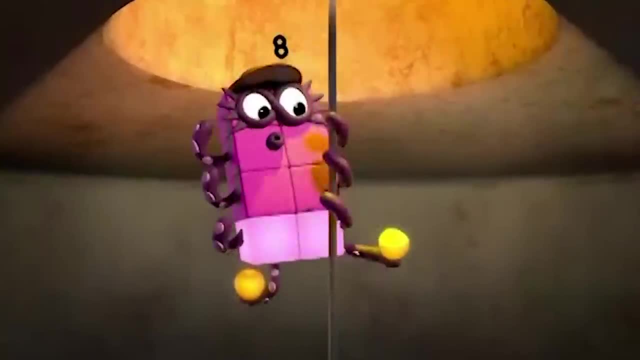 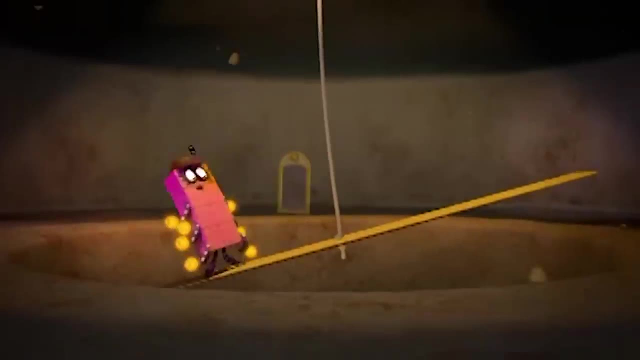 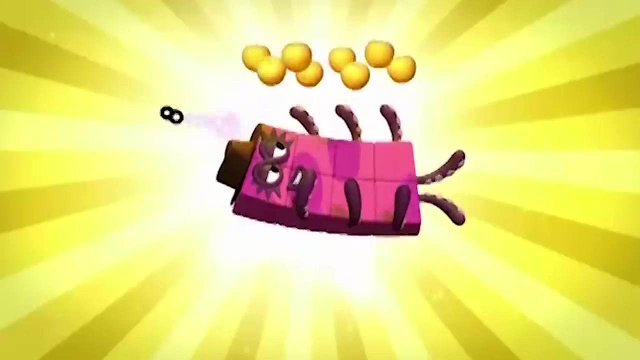 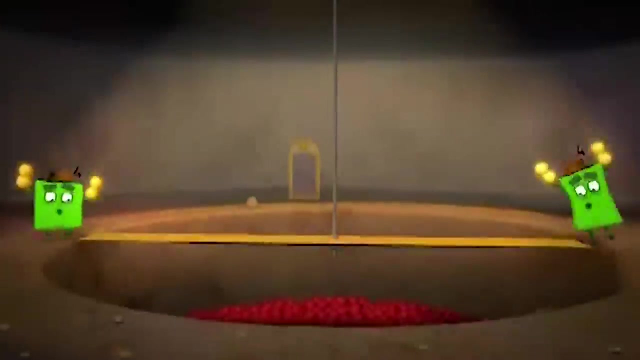 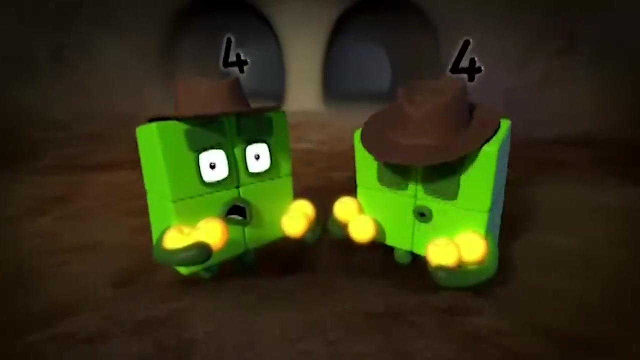 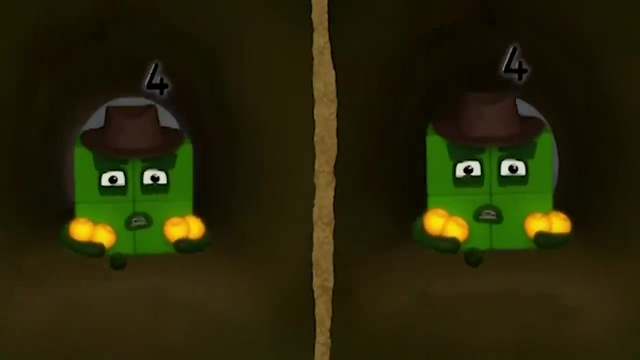 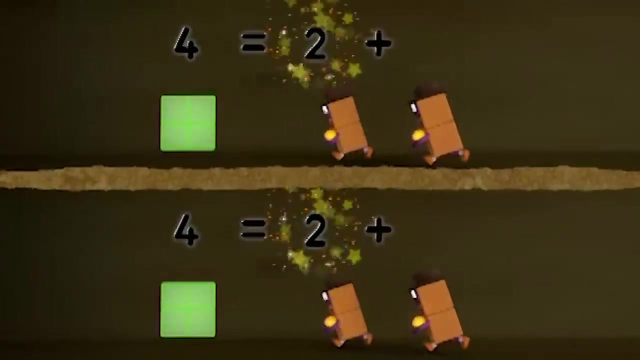 Time for a quick exit. Two, three, four, five, six, seven, eight. Octoblock splits in half Eight equals four plus four. Giant road thing alert, Look out River sneaks. Split in half Four equals two plus two. 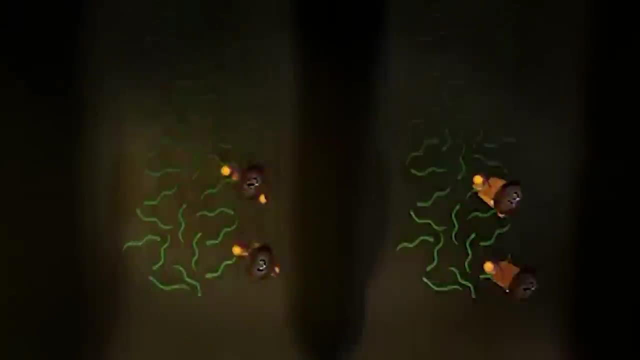 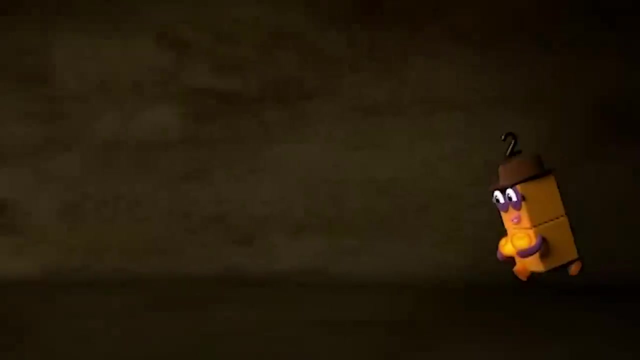 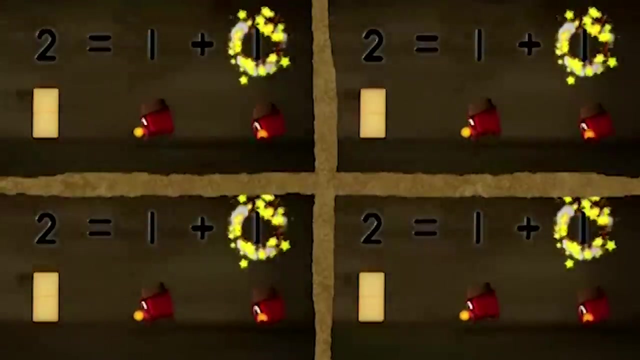 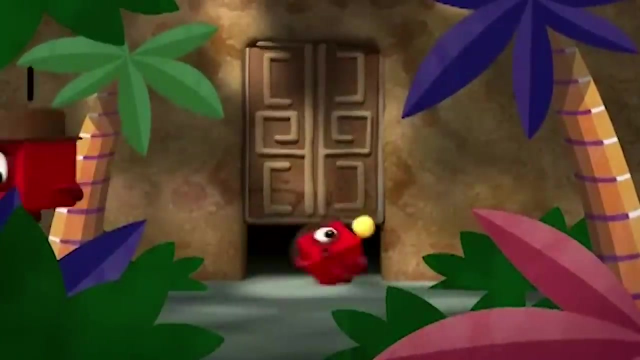 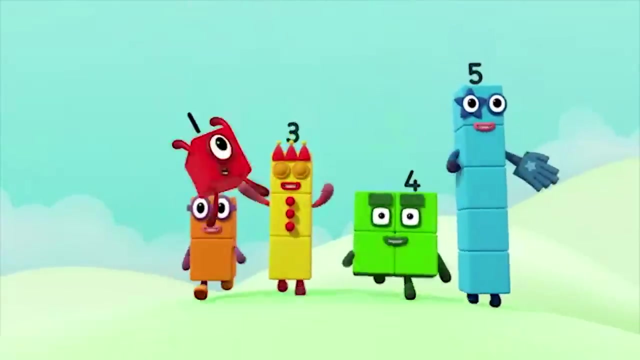